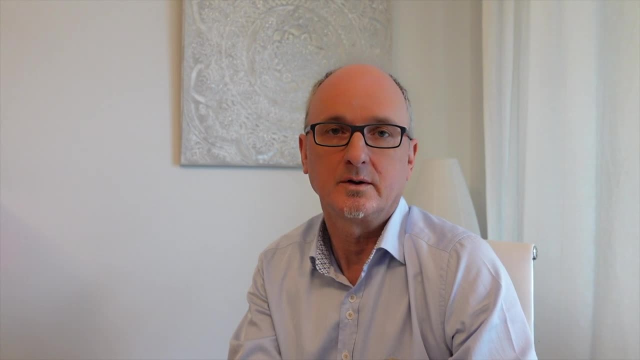 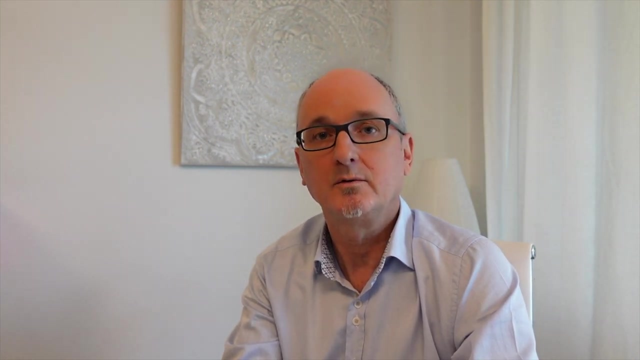 and I've got a graduate civil engineering degree. I have worked as a structural engineer for over 30 years now And my goal is to be a civil engineer. My motivation always was to put the following three things together in my work: First is the customer. 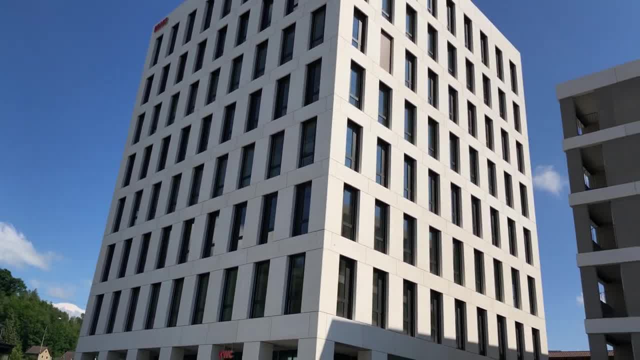 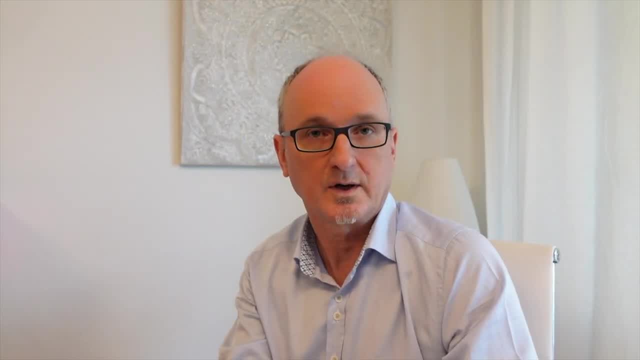 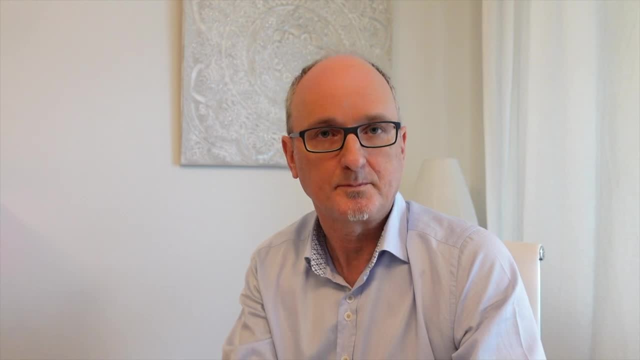 He pays the bills. He wants the construction of his needs and he wants it as economically as possible. Second thing is the construction site. You can design the greatest construction. If it can't be implemented on site, it's worthless. Third thing is the codes and the regulations. 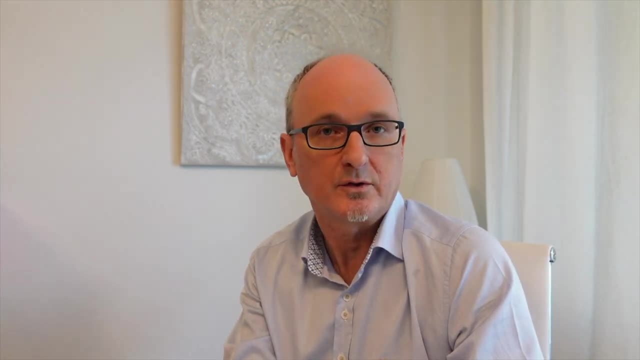 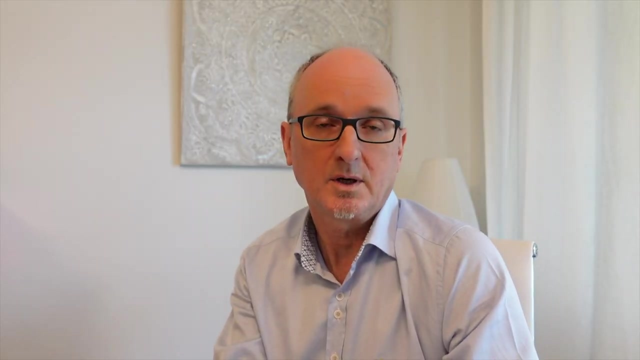 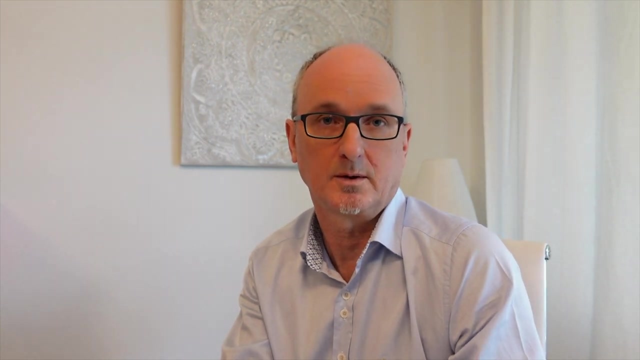 Of course you have to follow the local regulations and laws. But remember, an engineer is educated for and is meant to think by himself to find the proper solution for his specific problem. So do not rely on rules and codes, only Think by yourself. 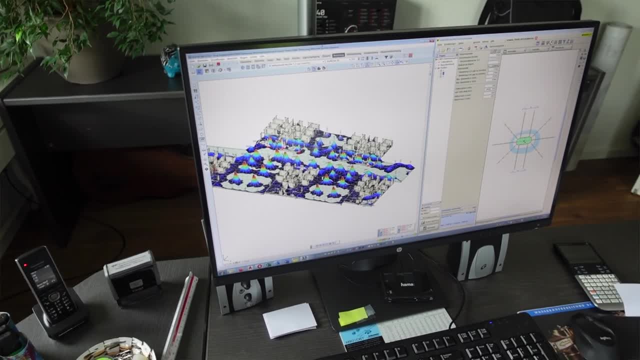 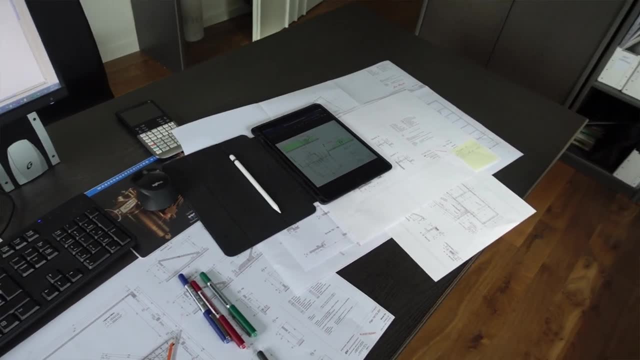 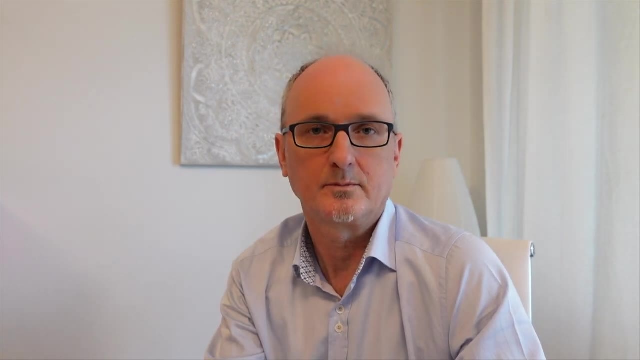 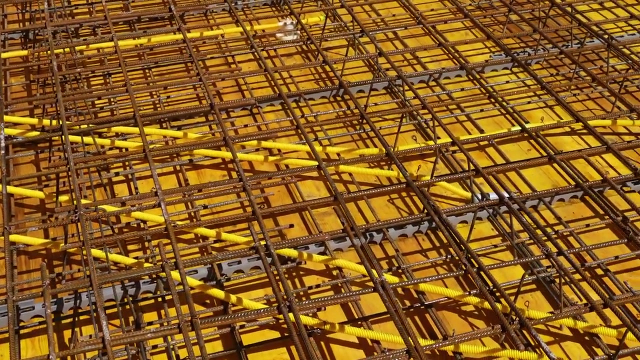 I run my own engineering company in Switzerland. What my team and I do is design and calculation of structural constructions. The most common construction in this country is a massive construction That's reinforced concrete and masonry. We use it for residential buildings and commercial buildings. 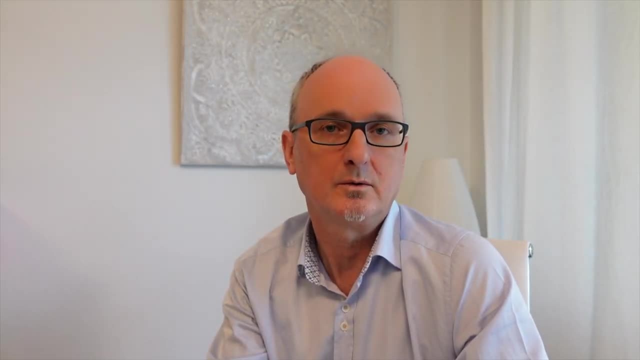 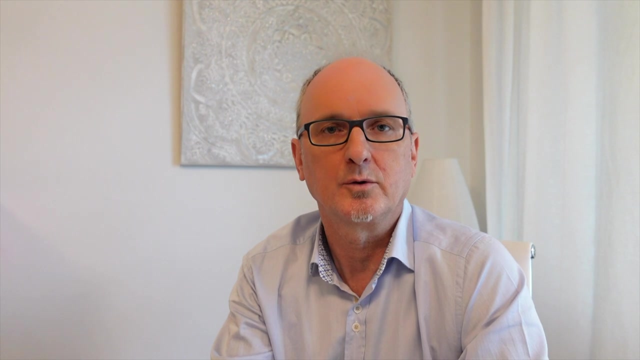 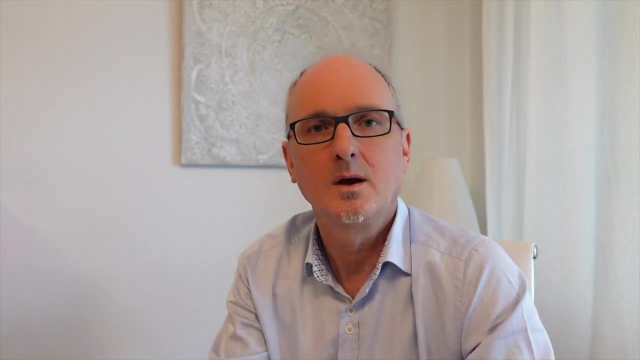 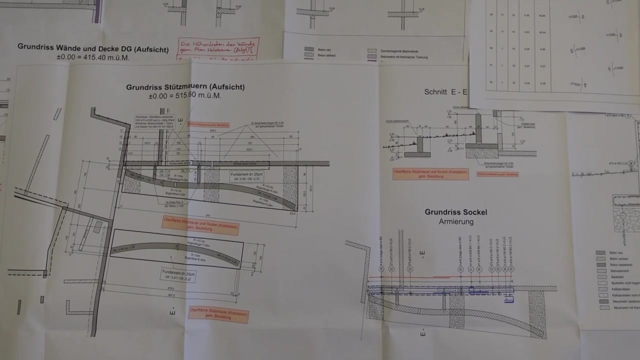 Usually it's the most economic way to construct and to build in this country. For industrial constructions like production halls, we also use steel structures or timber constructions. We provide the documents for the executing company on site, like the builder. These are the plans for formwork. 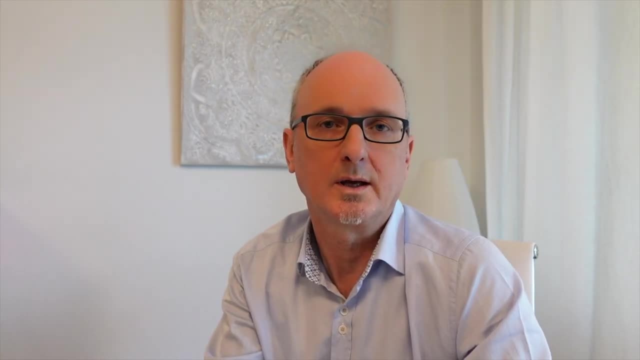 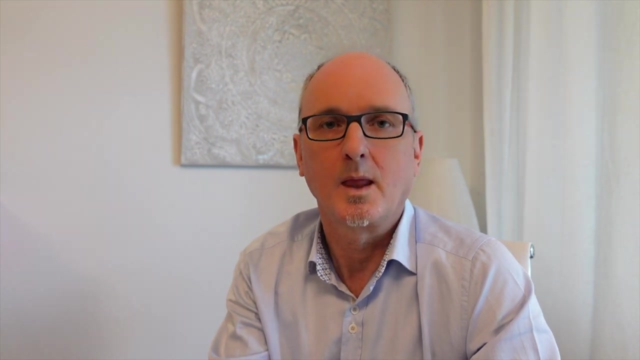 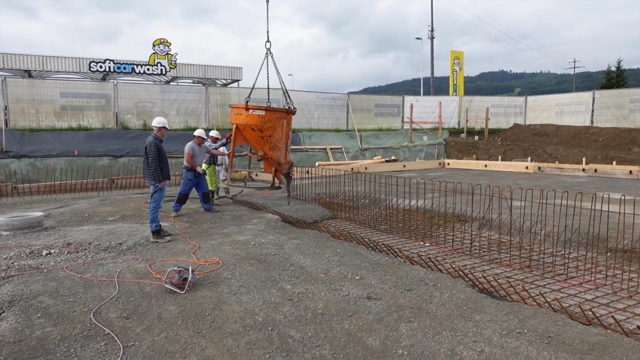 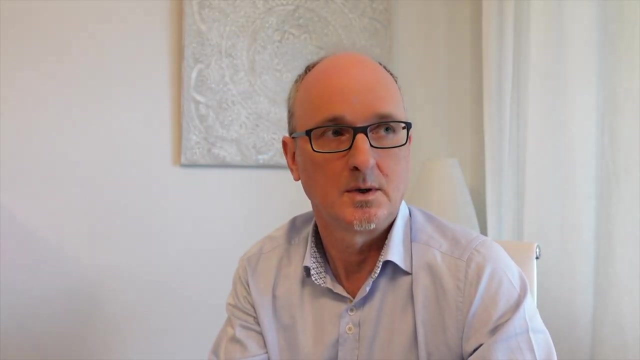 for reinforcement and also the belonging order lists. So we do not build the constructions ourselves, We just do the planning and the design and the supervision on site. For that we work in a team with the sanitary, with the airing, with the heating engineers.